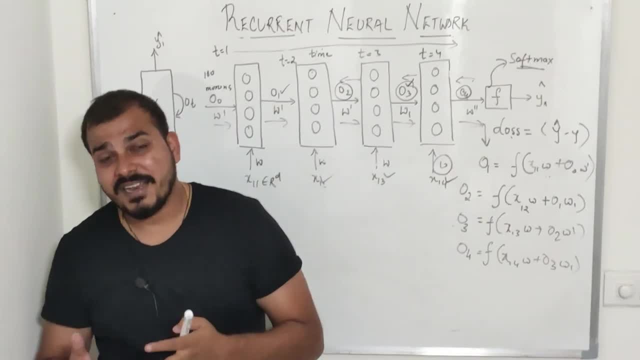 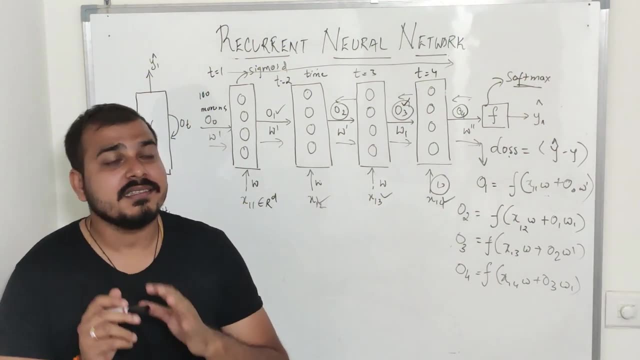 you a small idea about what is vanishing and what is vanishing: gradient problem and exploding gradient problem. Now let us understand what is the problem over here. So when we consider this hidden layer, there are neurons inside this particular layers, right, and we know that we. 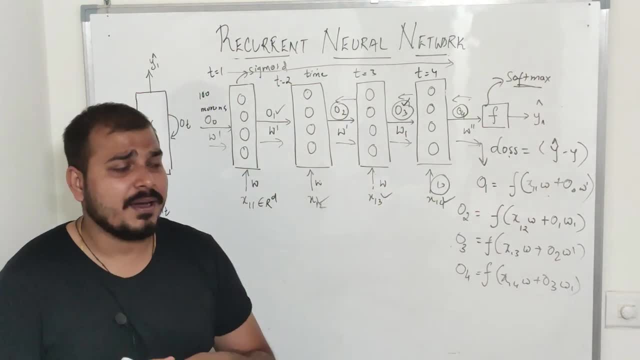 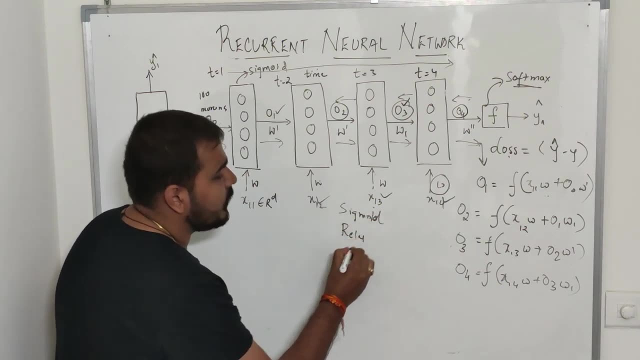 apply an activation function and most common activation function that you basically apply is like sigmoid right. It is like ReLU right, ReLU activation function. Now, understand what is the vanishing gradient problem. Now, guys, all the time when we do a backward propagation with respect to this, 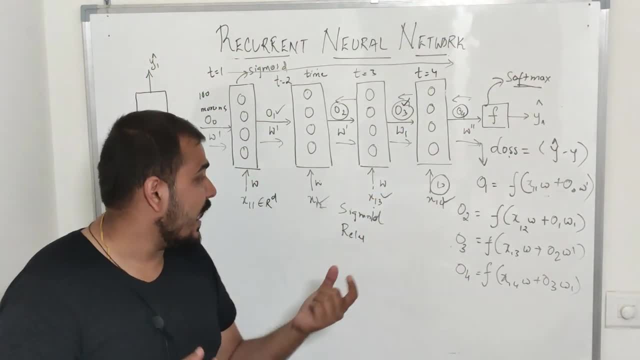 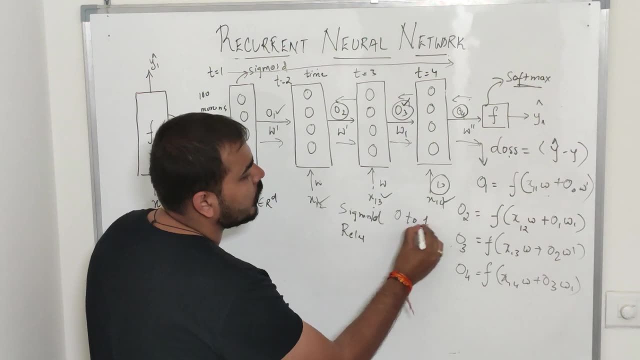 weights and if you have applied inside this neurons some activation function like sigmoid, if we find out the derivative of the sigmoid, it will always be between 0 to 1, always remember this Now, when it is between 0 to 1, now suppose over here we have calculated a derivative function. 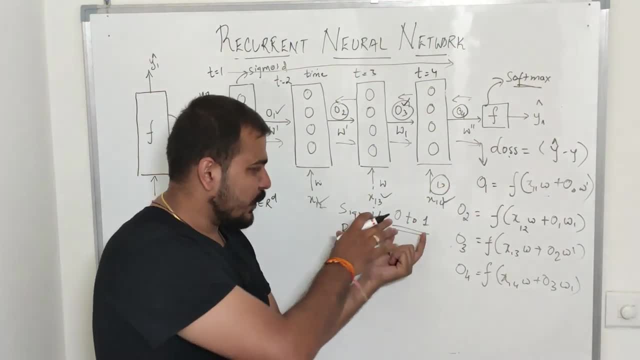 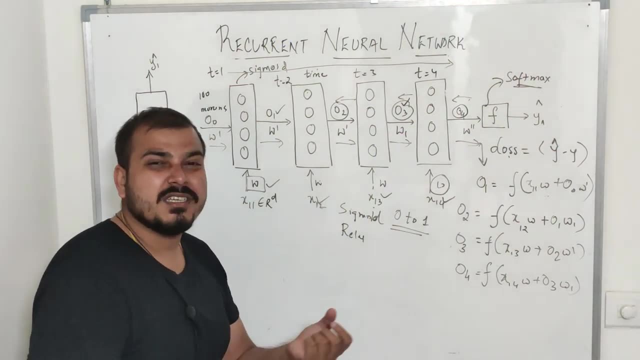 it will be between 0 to 1.. It will be between 0 to 1, right, So it is 0 to 1.. But as we go towards this W- Okay, towards this W- this value becomes a very smaller value itself, as the derivative is continuously happening, right. 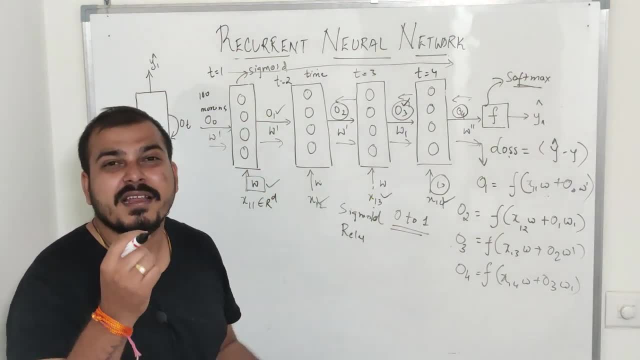 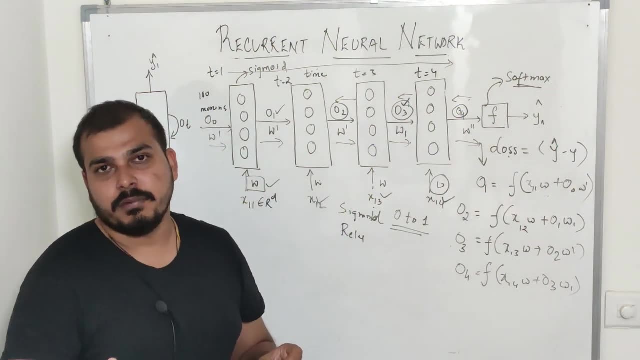 We find out the derivative of all this particular weights, This will become a very, very small value. now, when it becomes a very, very small value, Whenever we do an updation of this particular weights, it will be negligible, you know. and when it is negligible, 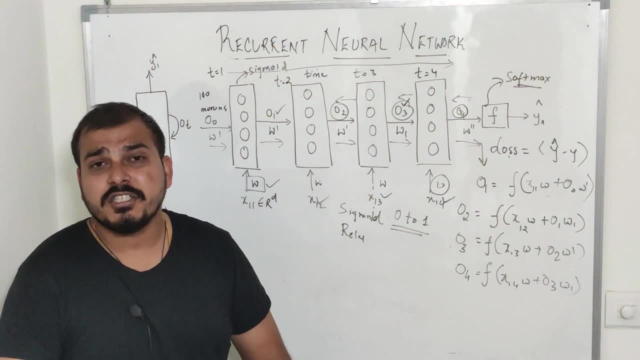 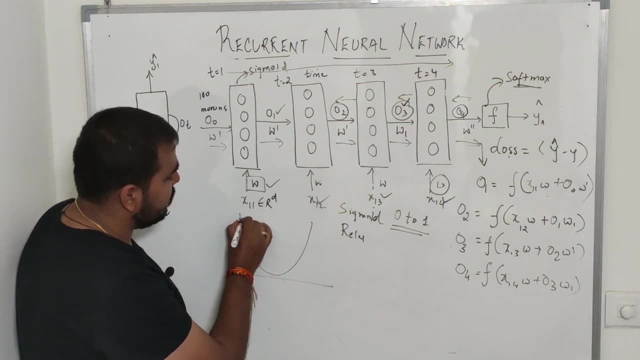 We will never converge or it will never converge to the global minimum point of a gradient descent. So if I gradient descent is like this right now- suppose this is my initial point- There will be a small movement over here again I'll be coming here, but it will never reach at this particular point. 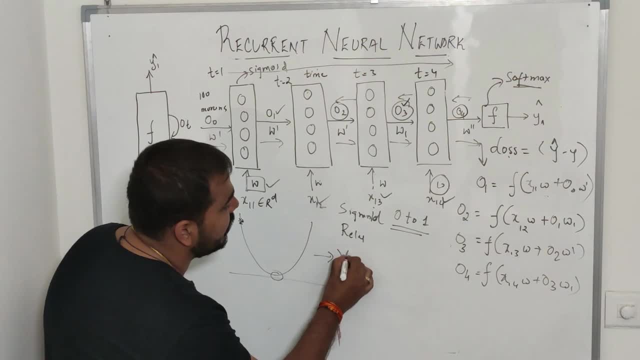 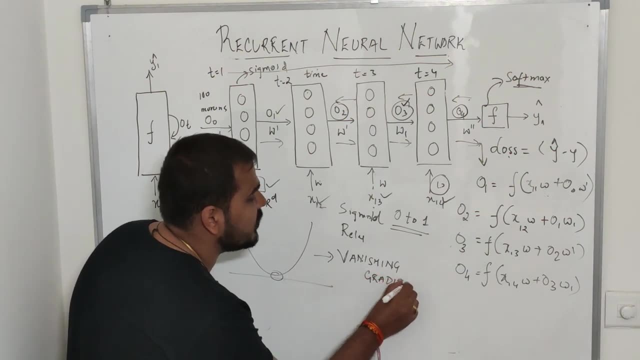 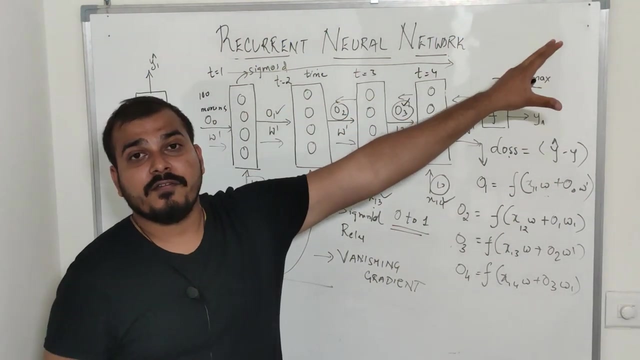 You know, because of that, this is basically called as vanishing gradient problem. vanishing gradient problem, Okay, that basically means that, suppose, if you are using some sigmoid activation function, And this is not happening because of the number of layers, It is just happening because of so many number of times We are actually running this back propagation. 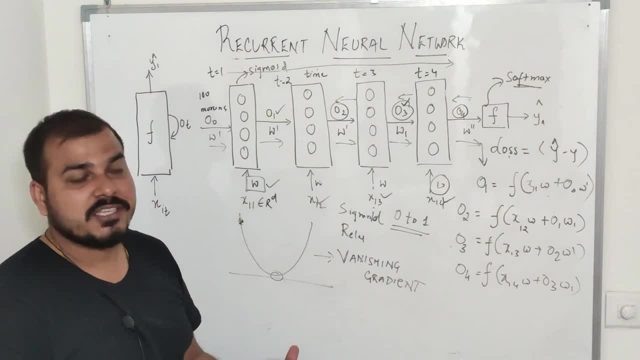 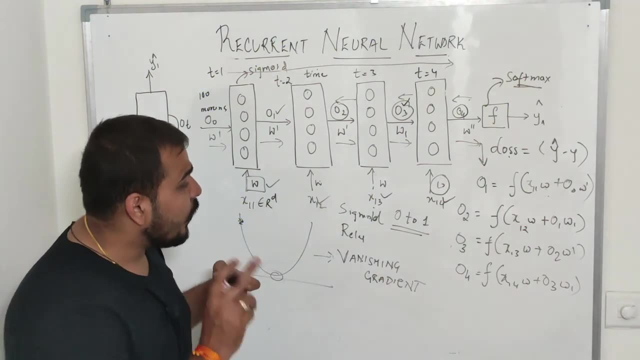 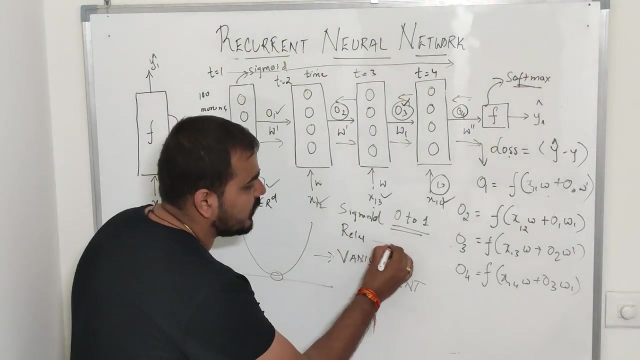 And as soon as we are updating this weights, this will actually create this vanishing gradient problem. We're in wherever this weight changes are there, It will be very, very negligible. Okay, Now there may be one more problem with this. you know, If you are using other activation function which is other than sigmoid, like a relu activation function, and suppose my derivative is greater than 1. 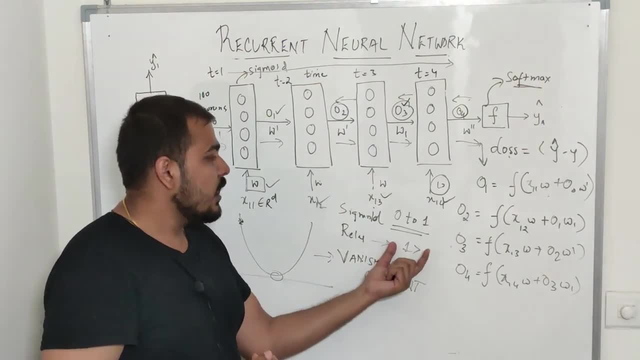 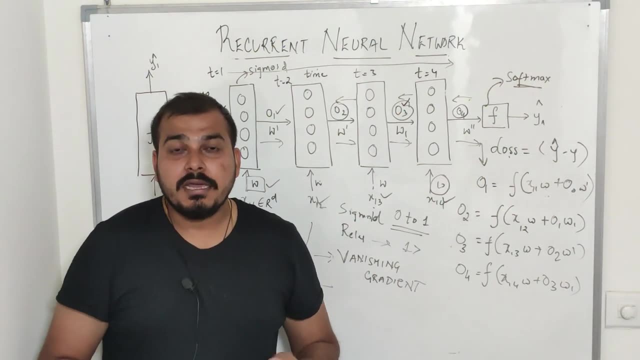 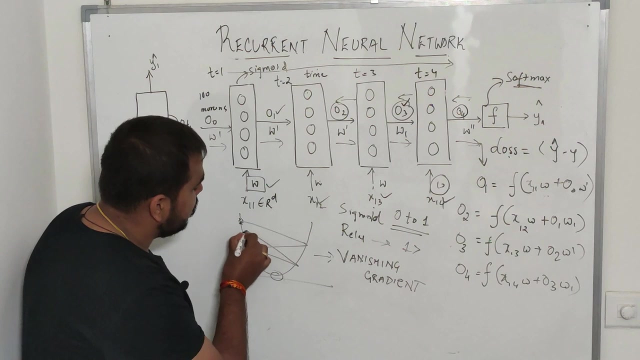 Okay, and it may be that we'll be getting so many derivatives later on with greater than 1, So as we go ahead towards this, it creates an exploding gradient Problem. you know, exploding gradient problem basically means that this W Changes will happen so big that it will never reach the global minima. It will be rotating here itself. 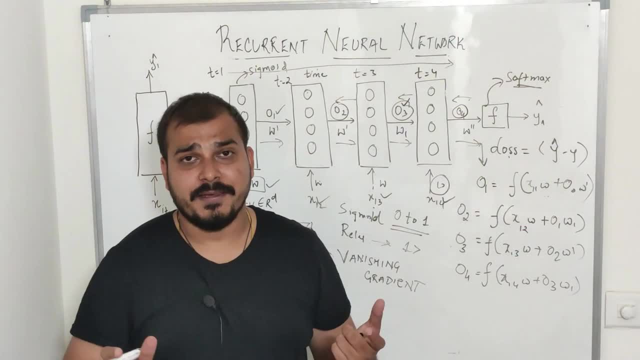 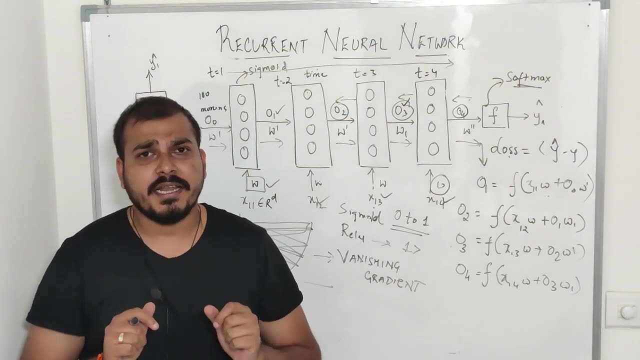 Okay, because the value of the change of W is very, very high. It will never reach this global minima. So, because of this particular problem, we use a simple architecture which is called as LSTM, that is, Long short term memory. we use this particular architecture. 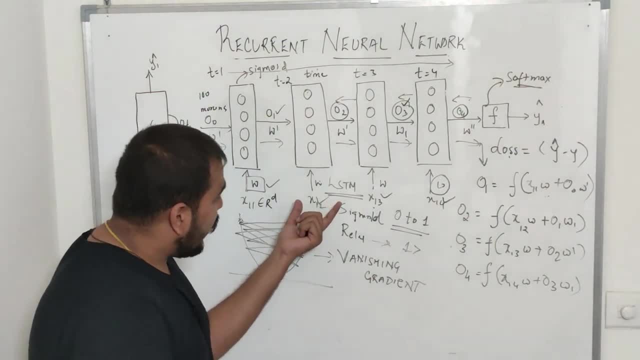 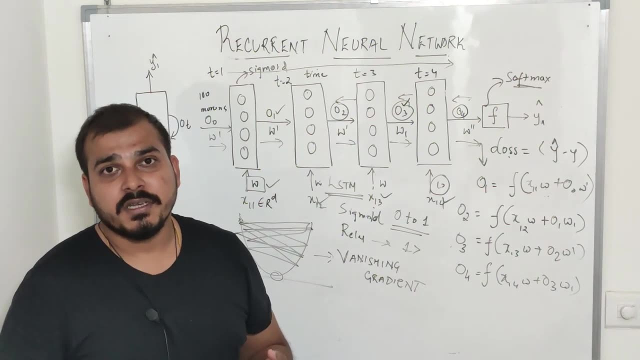 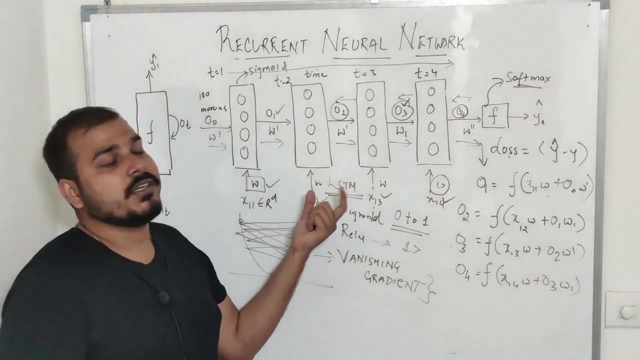 In order to solve that particular problem, now, When, and again. I tell you what is our LSTM, how it is different from a simple RNN in my upcoming videos. okay, but just understand that in order to solve vanishing and grade, vanishing and Exploding gradient problem, We use a structure called as LSTM, RNN, That is, long, short term memory recurrent neural network. again. 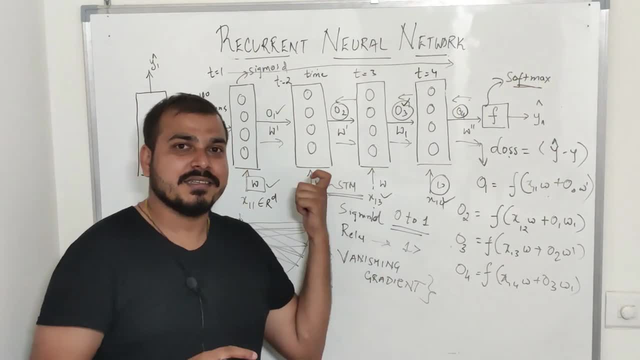 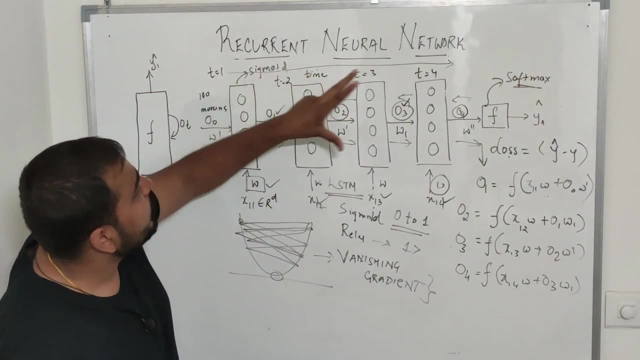 There is a small architecture difference between this particular RNN, a simple RNN, and an LSTM RNN. that I'll be discussing in my upcoming videos, but i hope you understood that. what is the problem with a simple r and n? understand, guys, as we are doing back propagation with respect to this particular time. 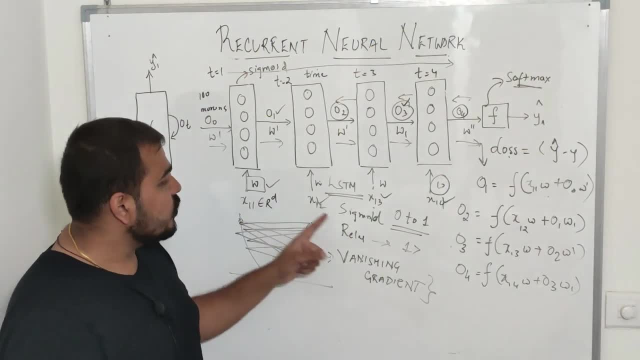 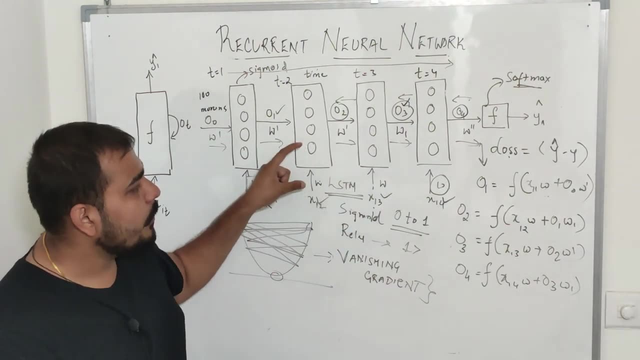 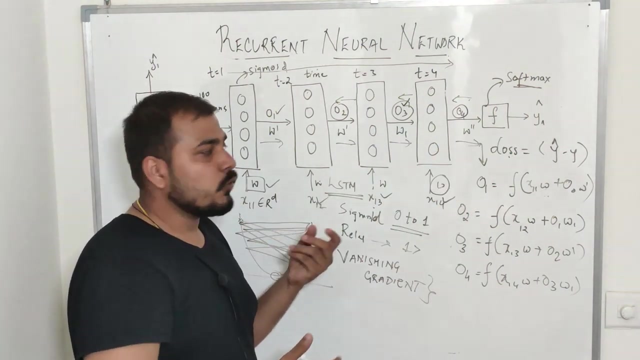 right. so when we reach over here and suppose, if you have used sigmoid activation function everywhere, right, and we know that the derivative of sigmoid activation function is 0 to 1, so every time we go back right the number becomes very small. suppose i have a sentence which is of 20 words over here. 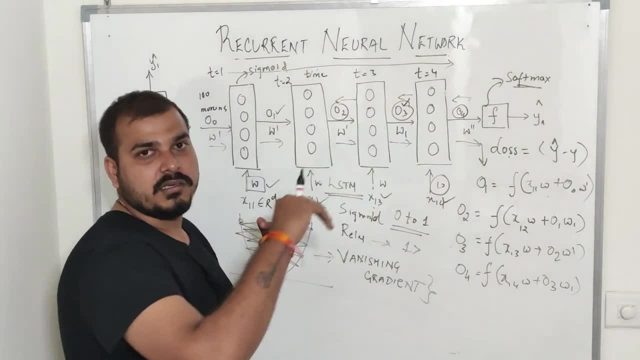 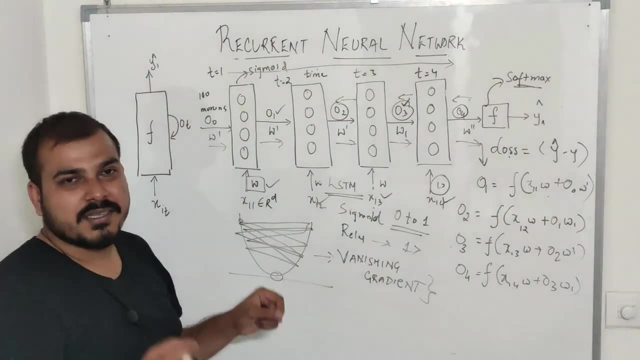 i have just drawn, t is equal to 4. suppose i have a sentence of 100 words, so my this value will increase to. t is equal to 100, right? so when we are doing the back propagation, this updates of this particular weight in at time is equal to 1 or time is equal to 2 will be very, very negligible and 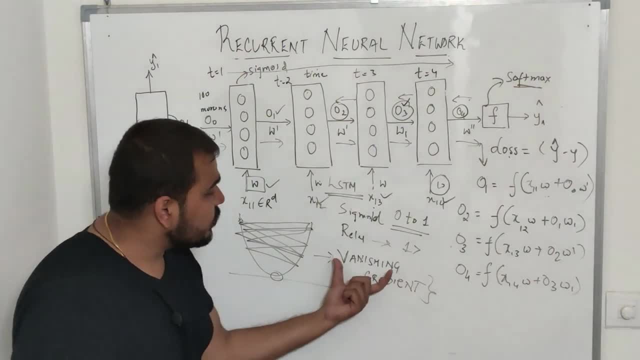 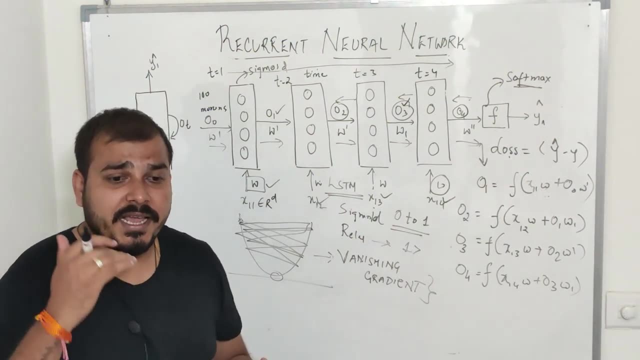 because of that it will never reach the global minimum. and similarly in the exploding gradient problem. what will happen? suppose we are not using- we have used other activation function other than sigmoid. then what will happen is that every time when we are updating this particular weights with the help of derivative